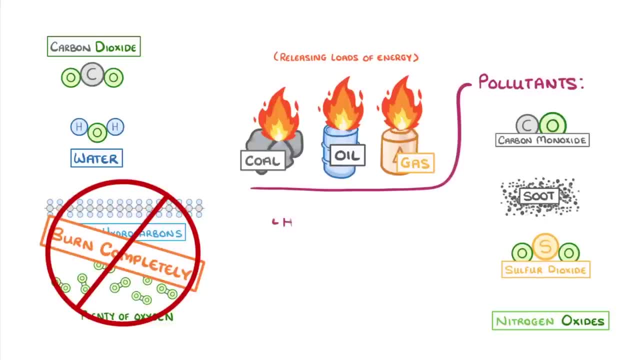 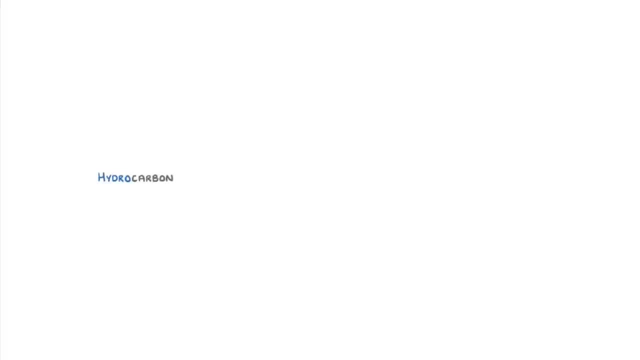 dioxide and nitrogen oxides, with a focus on how they're made and why they're harmful. Whenever a hydrocarbon burns in plenty of oxygen and so burns completely, we call the process complete combustion, And the only products we should get are water and carbon dioxide. However, when there's 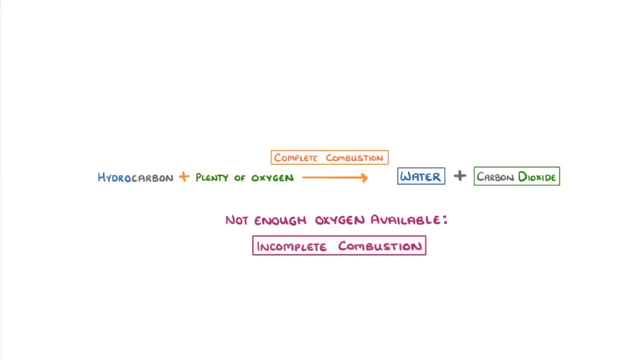 not enough oxygen available, we instead get incomplete combustion, which can release carbon monoxide, and particulates, which are solid particles of carbon that we call soot. If we start with particulates, there are two main problems that we have to solve. One is: 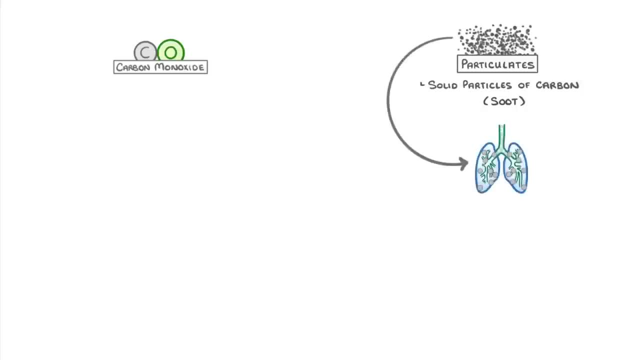 that they can get stuck in your lungs and damage them, which can lead to respiratory problems. The second issue is that they can form dark clouds or smog, which reflects sunlight back into space, and this means that less light reaches the earth, which we call. 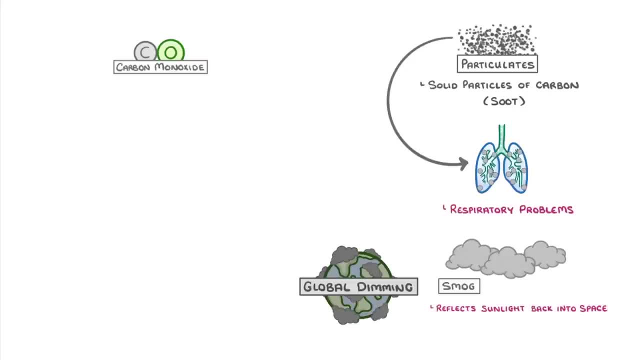 global dimming. Carbon monoxide, on the other hand, is dangerous for one very specific reason. If we breathe carbon monoxide in from the air, it diffuses into our blood and binds to our haemoglobin in the same place that oxygen binds. This means that our haemoglobin 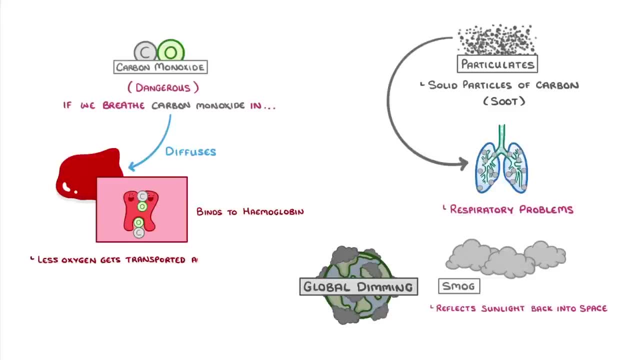 can carry less oxygen, and so less oxygen gets transported around the body. In severe cases, this can lead to fainting, a coma and even death, as our brain becomes starved of oxygen. And to make things worse, carbon monoxide can also cause a lot of problems, such as: 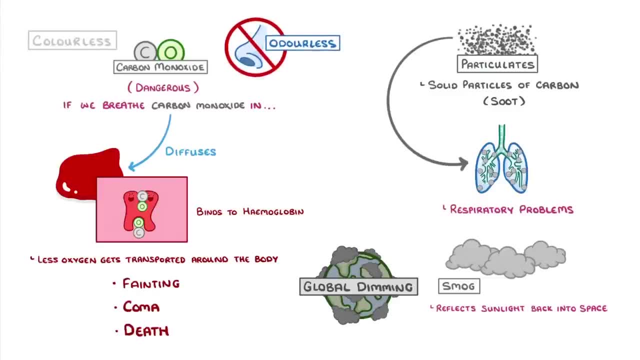 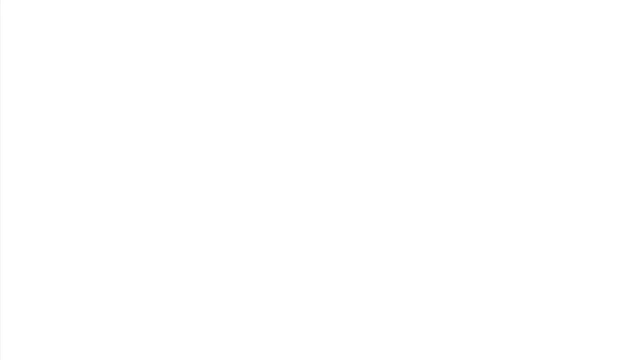 a high blood pressure. a high blood pressure and a high blood pressure. Carbon monoxide, however, is both colourless and odourless, which makes it really hard to detect. Pollutants like sulphur dioxide and the different nitrogen oxides, meanwhile, are made a bit. 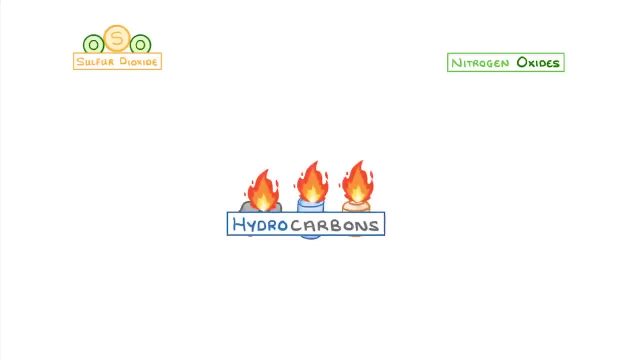 differently. Sometimes the hydrocarbons that we burn have impurities in them, like atoms of sulphur. So when we burn them, the sulphur gets oxidised to sulphur dioxide gas. Meanwhile, at nitrogen oxides we have a lot of impurities in them, like atoms of sulphur. So when we